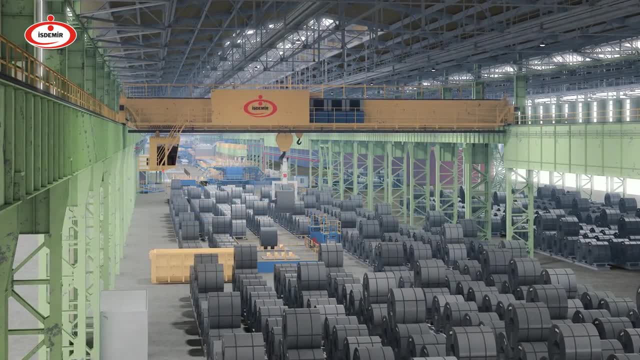 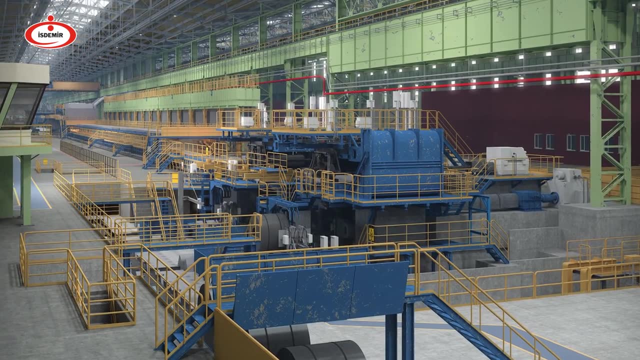 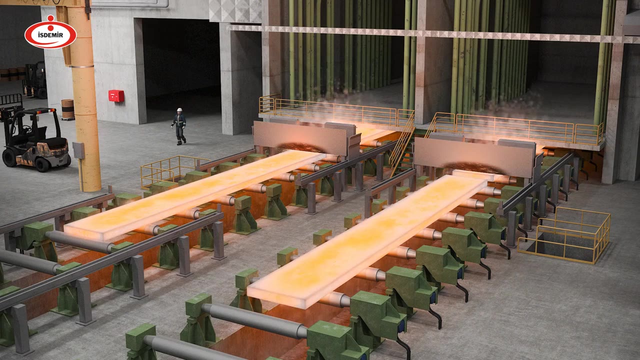 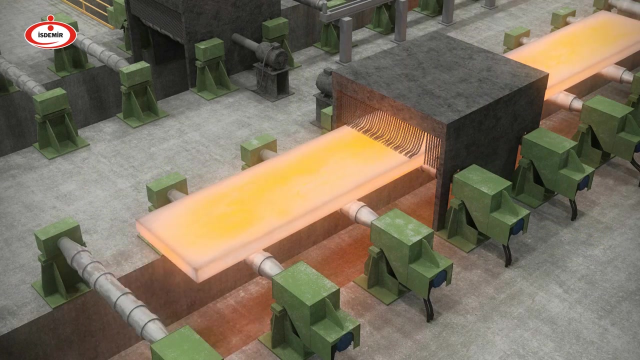 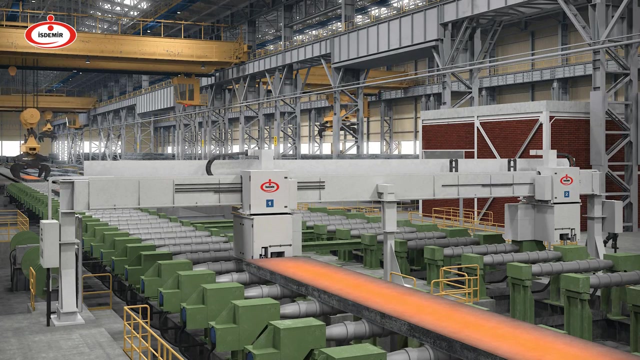 With its 3.5 million tons per year capacity. hot rolling mill precision alloyed lathes and liquid steel is solidified in slab caster according to product requirements. Slabs are systematically numbered for product traceability and are transferred to the stock area. 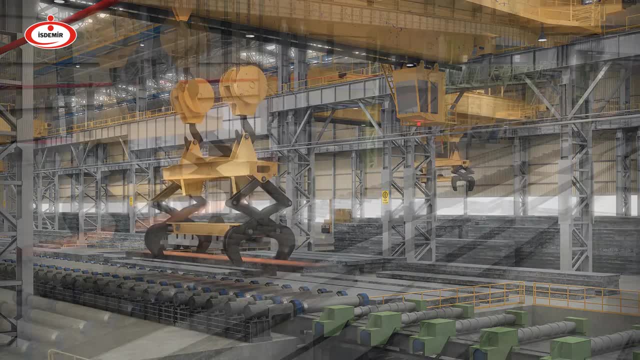 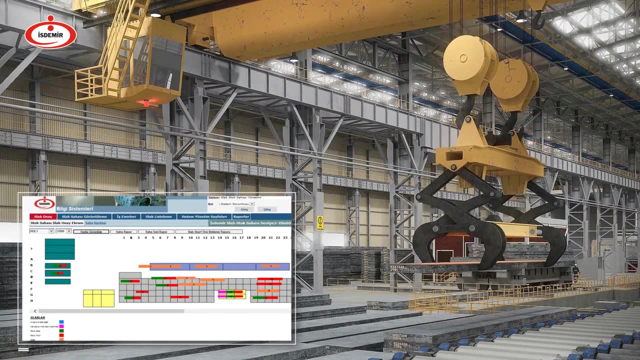 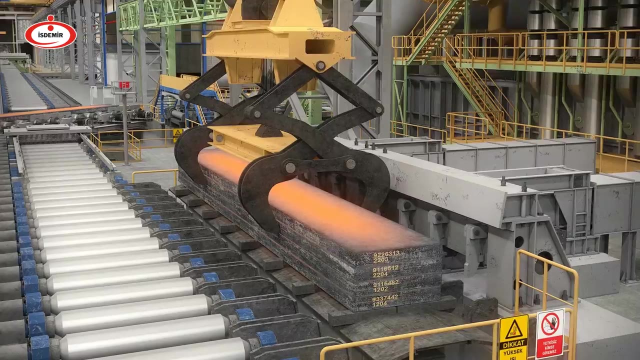 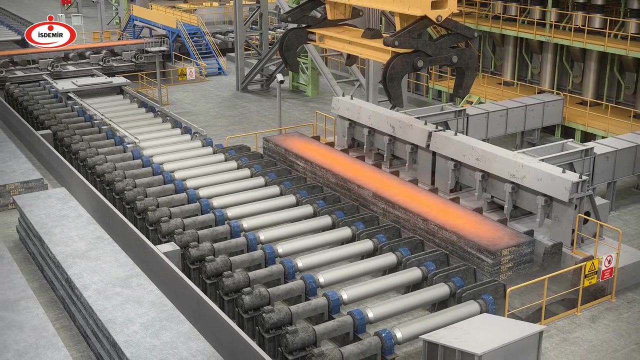 Slabs are stocked by numbering with slab tracking system. The number of each slab can be monitored in the slab tracking system through the stock field movements. Slabs are supplied to the reheating furnaces according to the production schedule by means of the overhead crane after the quality approval process has been completed. 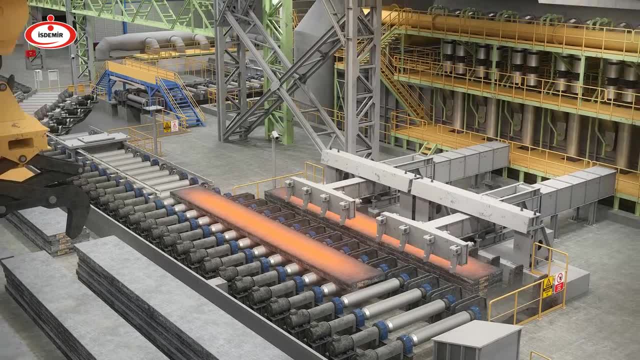 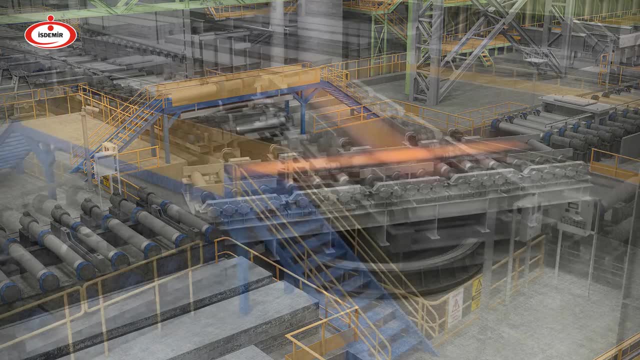 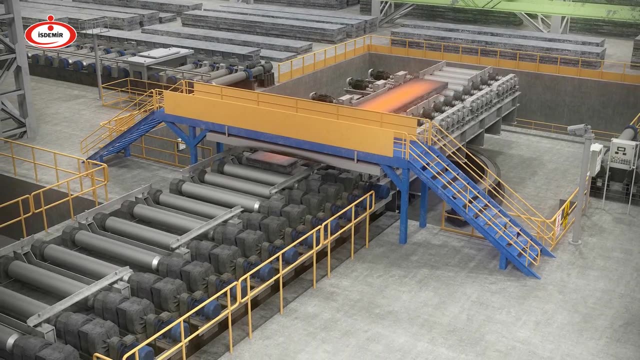 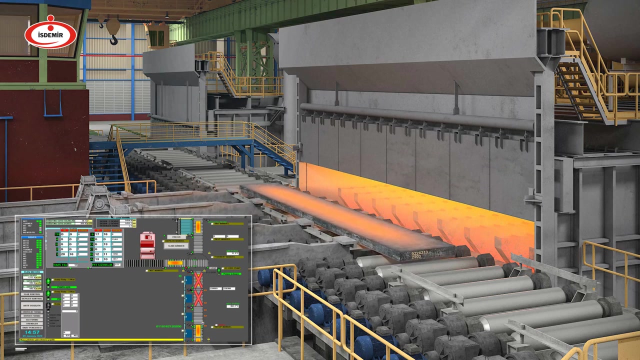 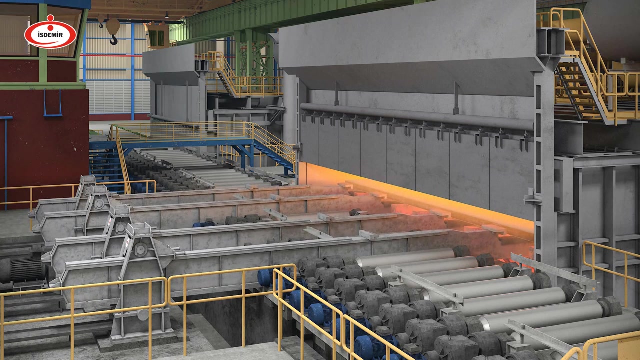 The number of slabs charged at the entrance to the furnace is checked by the number in the information system. They are heated to the required temperature for rolling, Using natural gas and coke oven gas. Different heating patterns can be applied according to quality requirements. 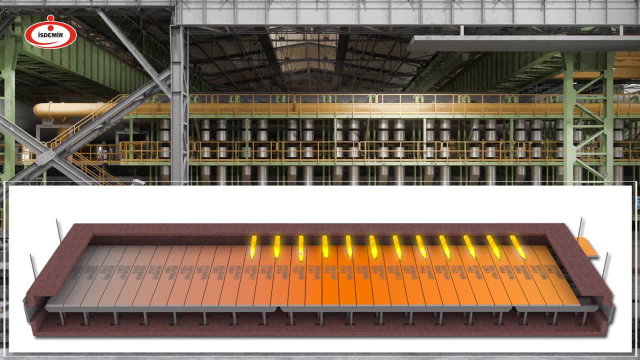 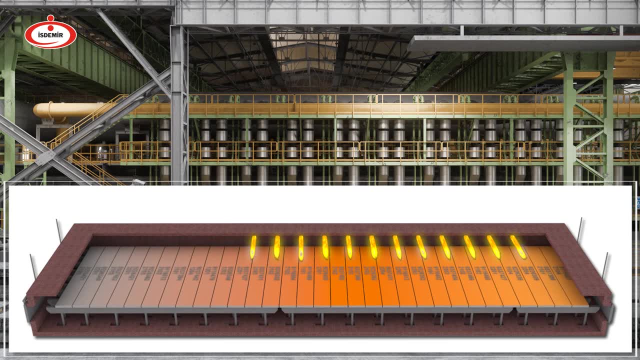 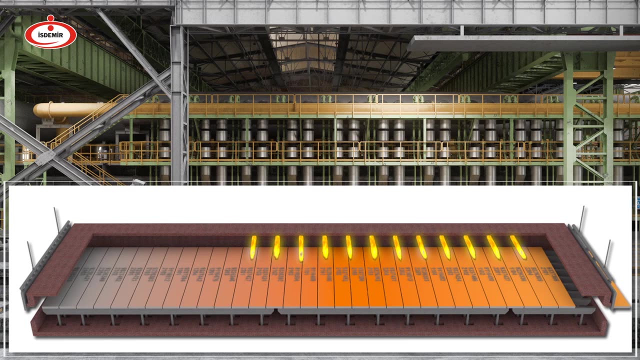 Two walking beam slab furnaces heat the slabs to homogeneous temperatures between 1100 and 1200 degrees Celsius. Slabs are prepared for the rolling process in fully automated furnaces by maintaining their surface quality. If the print is tentric, they don't need seasoning. 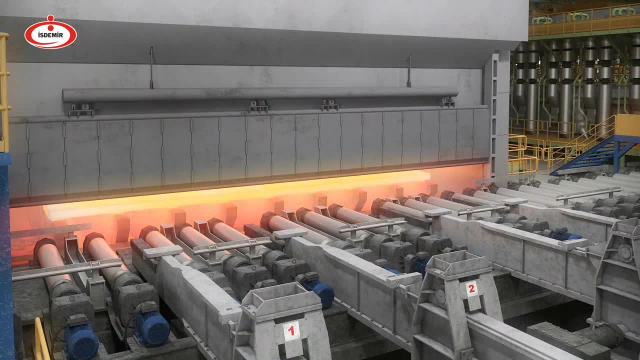 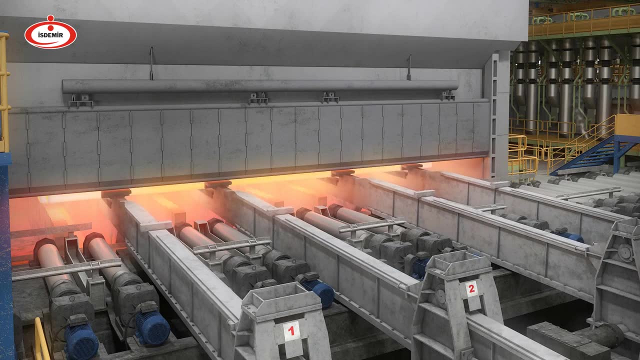 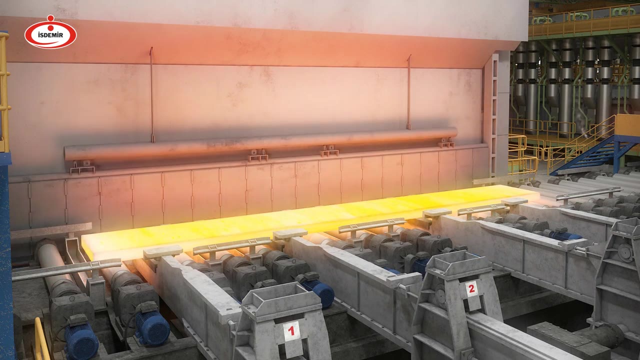 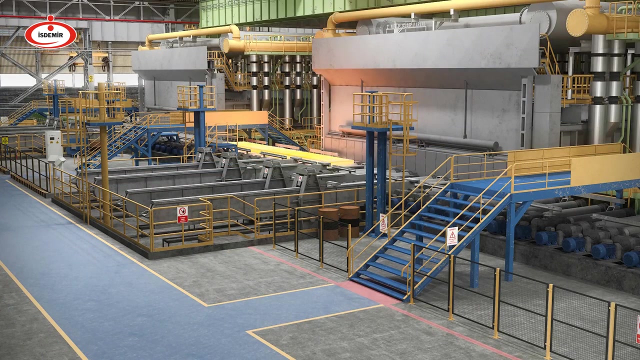 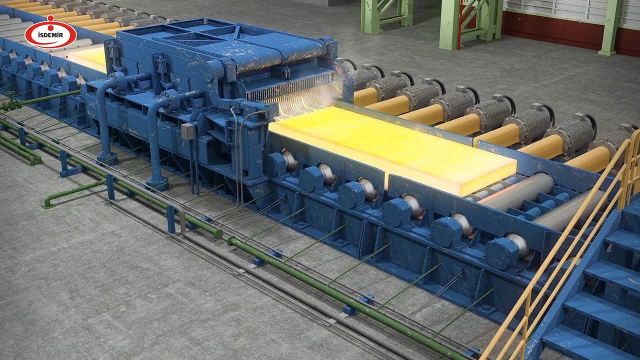 Or CPUs are stored inside the furnace to heat up fresh parts of the furnace In échelle небè raqe, raqe, raqe, raqe, raqe, raqe, raqe. by spraying high-pressure water. Effective descaling especially enables production of coils with high surface sensitivity. 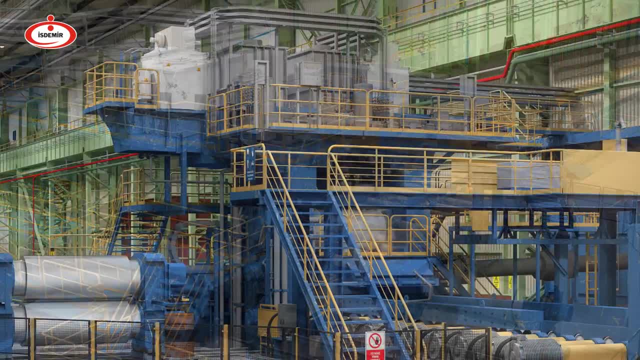 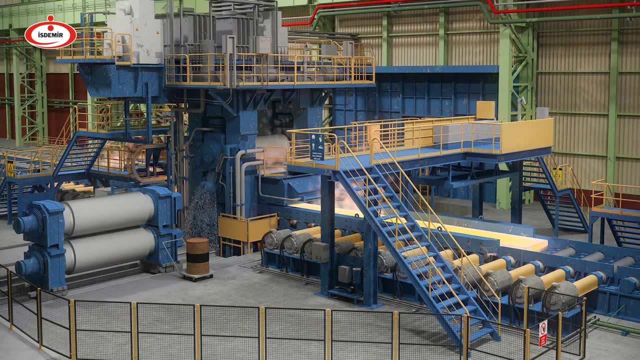 After descaling is done on the slab surface before strip rolling and rough rolling is performed in the rougher mill. slab thickness is reduced to 30 or 40 mm according to product quality, with 5 or 7 passes from 225 mm thickness. 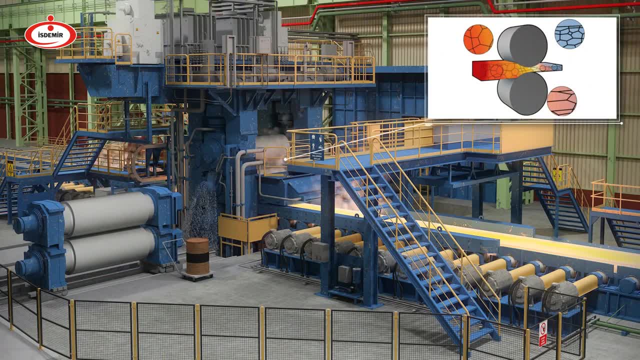 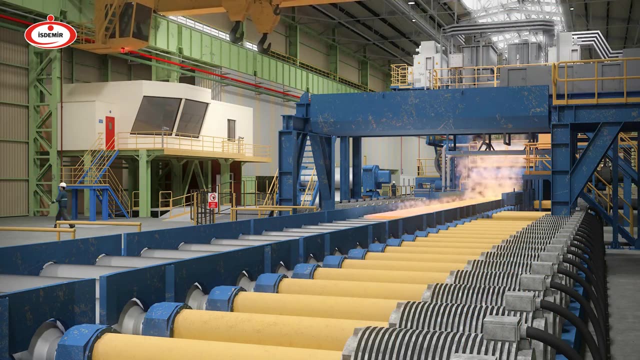 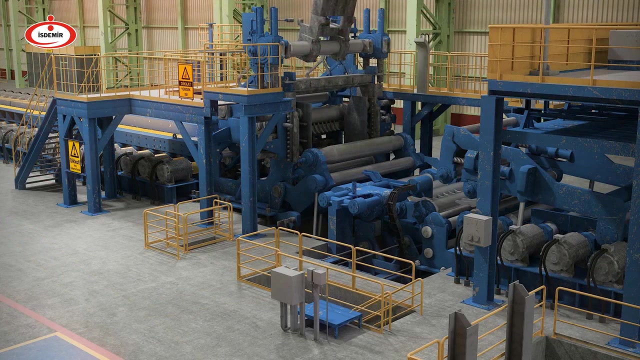 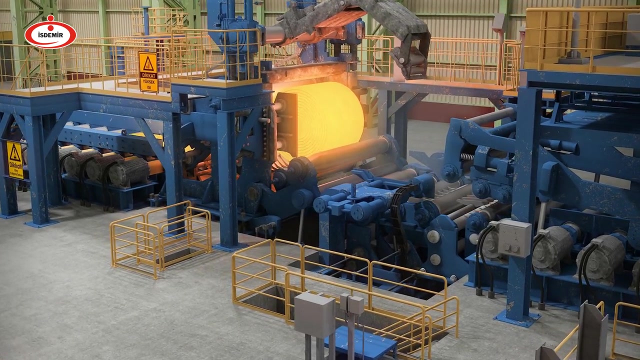 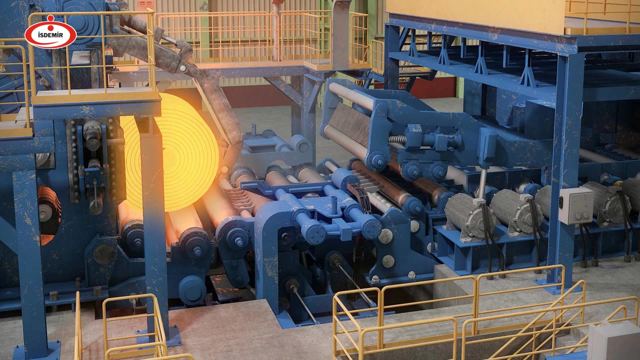 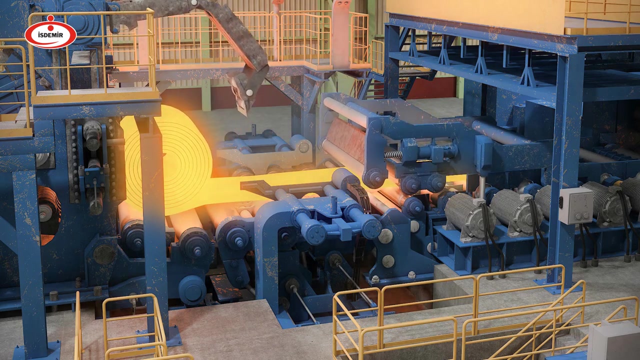 Working simultaneously with rougher mill. edger optimizes material width according to product demands. Coil box ensures a uniform distribution of the mechanical properties by keeping the temperature uniform throughout the coil. Uneven head and tip parts of the material are cut with a shear. 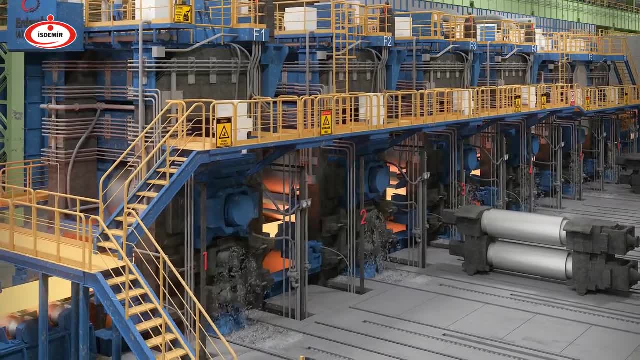 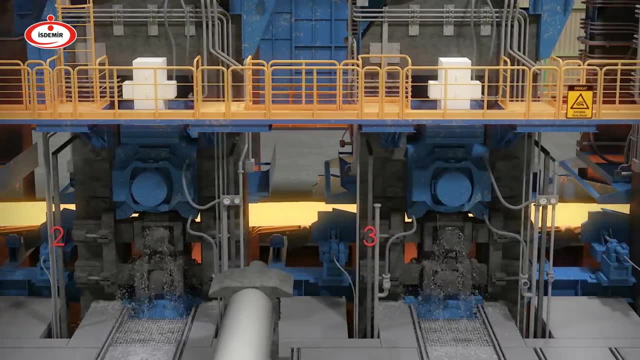 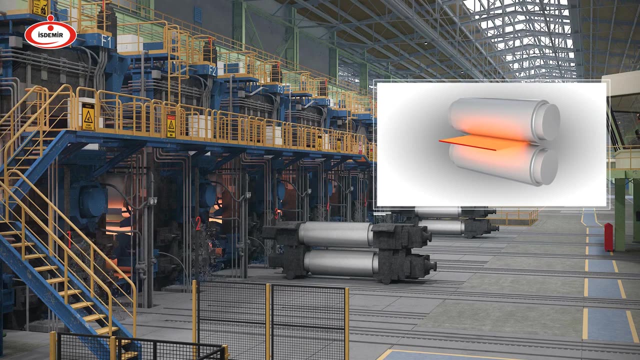 The product is finally processed to the final thickness with 6-stand rolling stand in the strip rolling section. Profile with special crown and thickness tolerances are produced In rolling mills. the profile structure that is suitable for specific uses is provided with roller crossing, bending and shifting features. 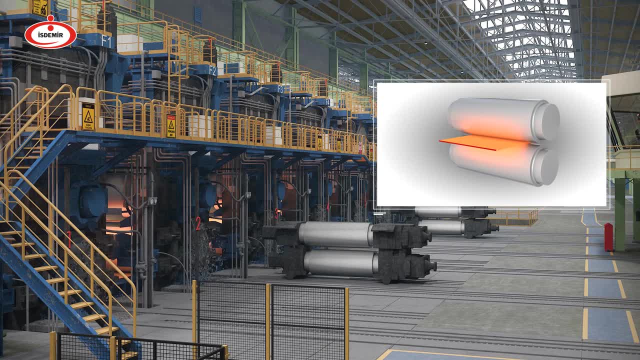 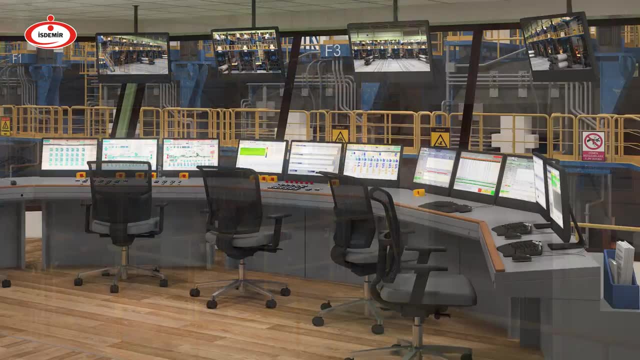 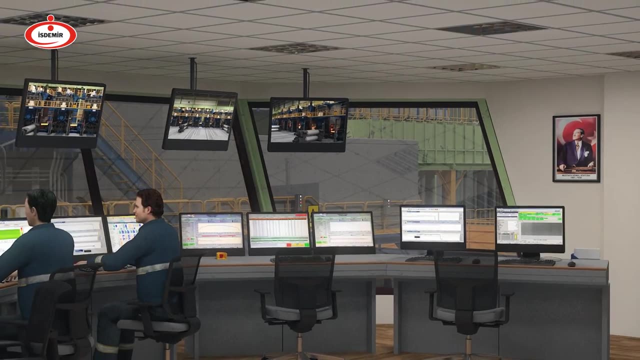 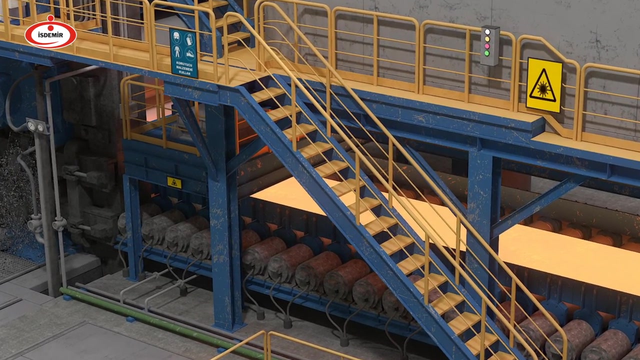 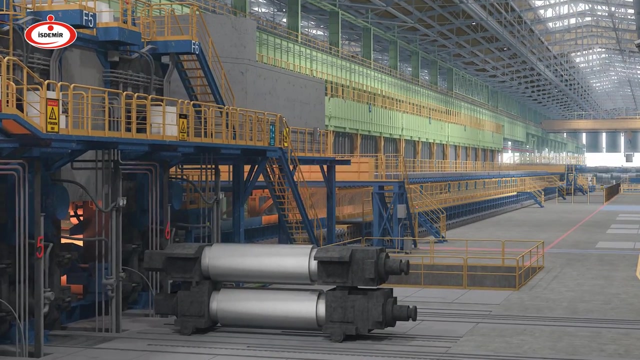 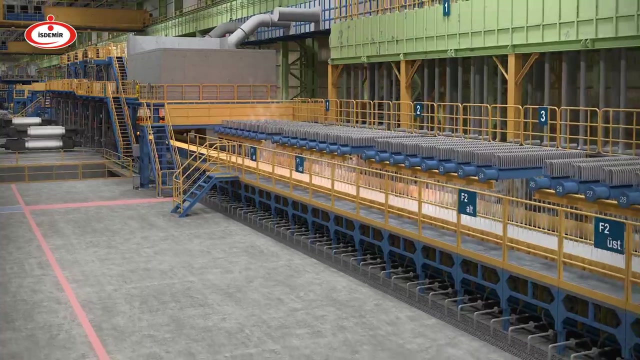 Instruction and Dimension profile along the coil is monitored by measuring the thickness and width of each point of the material. The upper and lower surfaces of each coil are inspected by the surface inspection system. Different metallurgical and mechanical properties are obtained by applying different cooling programs in accordance with the microstructure and mechanical properties requested for the. 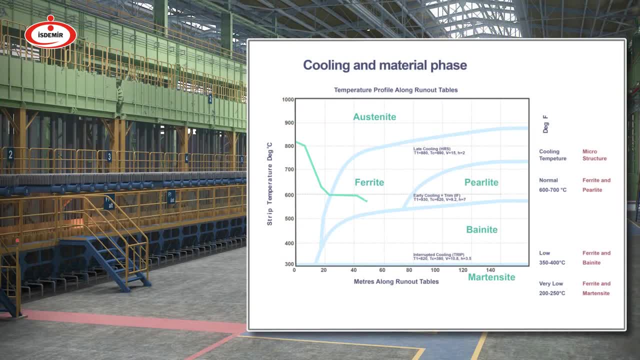 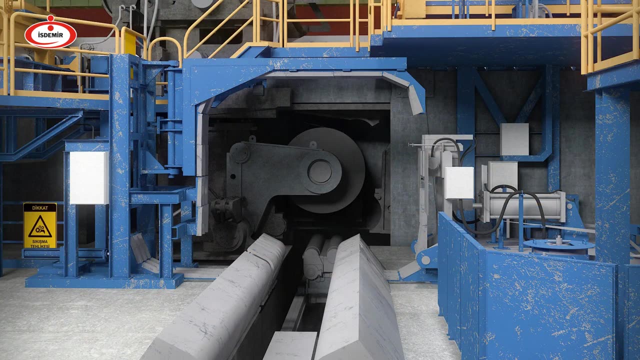 product. A wide range of products are produced from dual-phase steels with up to 300 different grades, including S700MC in HSLA group and X70 in API grades. The coils whose rolling process is finished are taken into the form of the coil by the